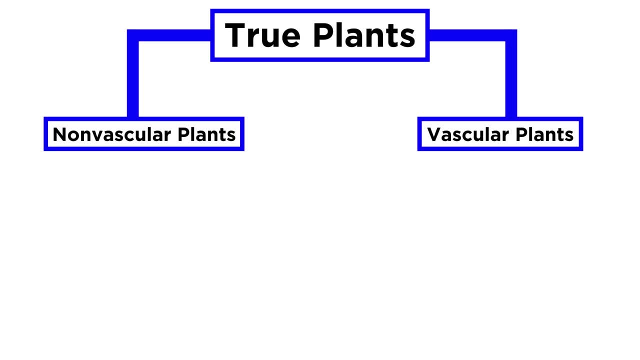 There are two different major groups of true plants. These are vascular and nonvascular plants. Nonvascular plants are usually small and relatively simple in their structure. This is because they lack the xylem and phloem vascular tissues we learned about earlier in the series. Without vascular tissues, these simple plants have no way to transport water. and nutrients long distances through the soil. So they're usually small and relatively simple in their structure. This is because they lack the xylem and phloem vascular tissues we learned earlier in the series. Nonvascular plants are usually small and relatively simple in their 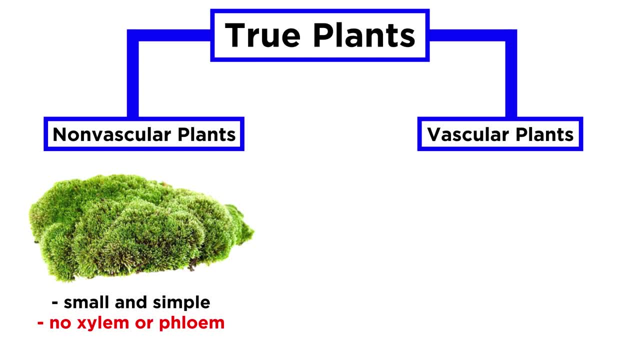 structure. This is because they lack the xylem and phloem vascular tissues we learned earlier in the series. So they lack the xylem and phloem vascular tissues we learned earlier in the series. So they don't have long stems or complicated structures Nonvascular plants also don't have. 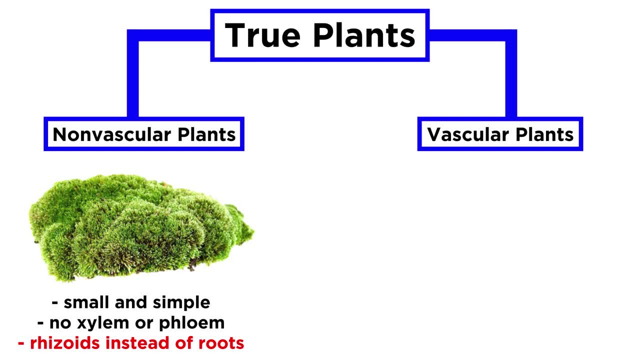 roots, but instead hold on to their substrate using tiny hairs called ryzoids. As you might expect, since their structures and reproduction are much less complicated, nonvascular plants are much older on the evolutionary timeline than vascular plants. Some examples of nonvascular 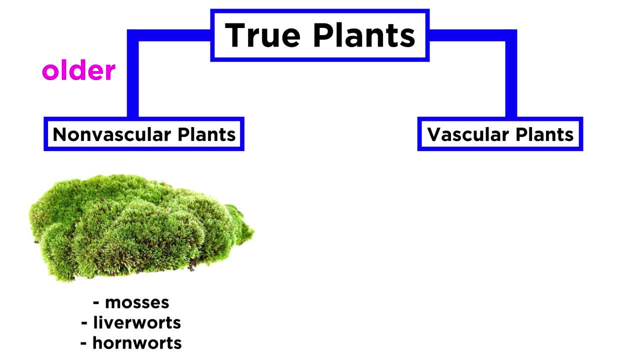 land plants are mosses, liverworts and hornworts. On the other hand, the more complex and more recently evolved vascular plants have complex structures. Vascular plants have xylem and phloem which, as we learned, facilitate the transport of. 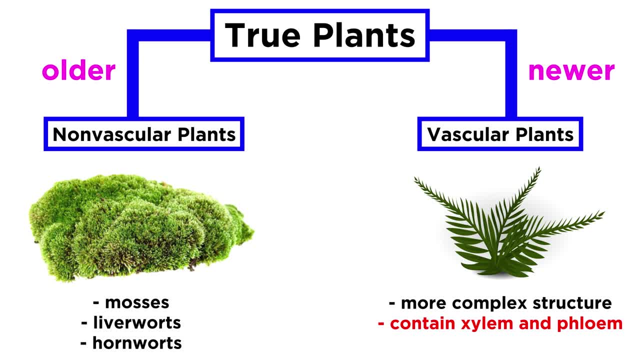 water and nutrients through a plant's body, allowing it to grow very large. These vascular tissues also allow for more complex structures like roots, long stems and branches. Examples of vascular plants include ferns, conifers and flowering plants. Now that we know the basic differences between vascular and nonvascular land plants, let's 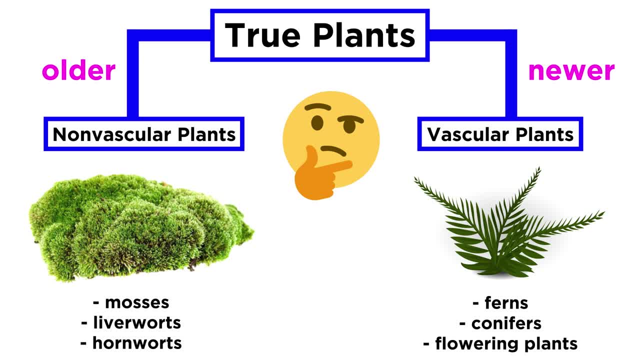 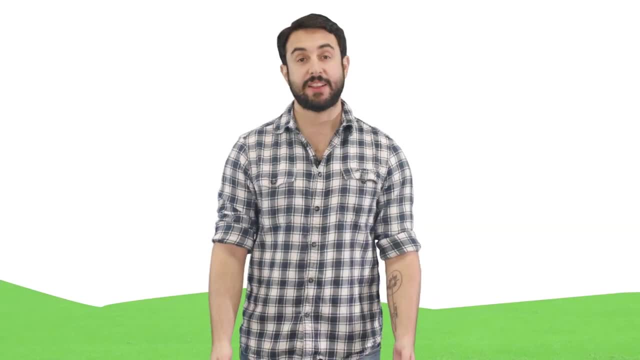 use the next few tutorials to take a closer look at these groups and specific types of plants within them, so that we can understand their structures and their reproductive systems, as well as how these different capabilities arose from an evolutionary perspective. Thanks for watching. 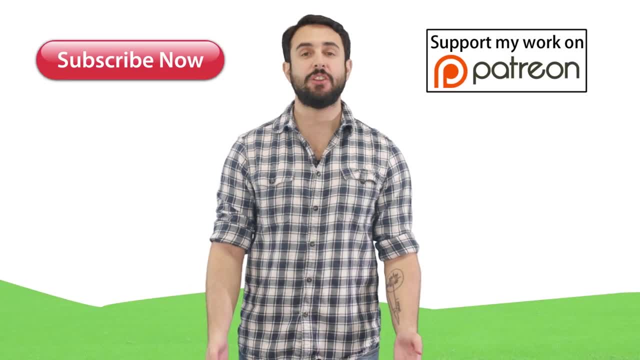 Subscribe to my channel for more tutorials. support me on Patreon so I can keep making content and, as always, feel free to email me professordaveexplains at gmail dot com.